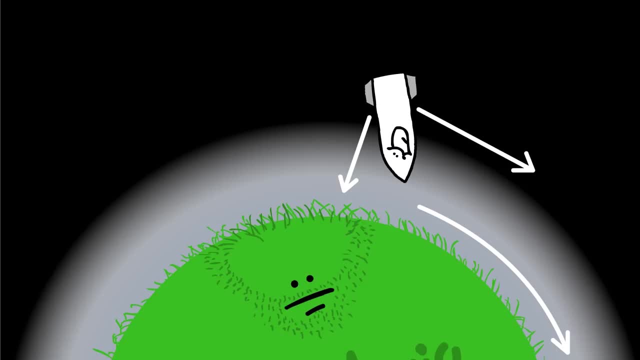 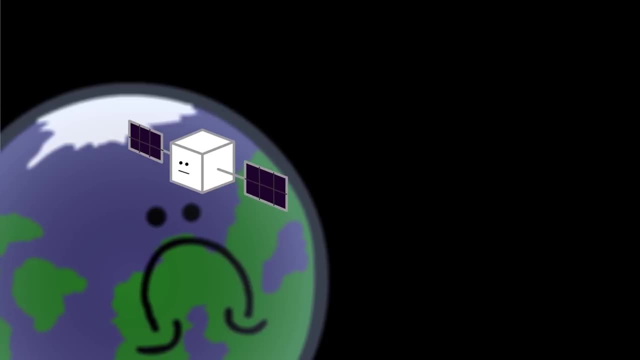 can hit it. Danny will stay like this forever if his velocity doesn't change. In the real world, this means the satellite can float around Earth endlessly without having to burn any fuel. This is all great in itself, but we're going to have to figure out how to. 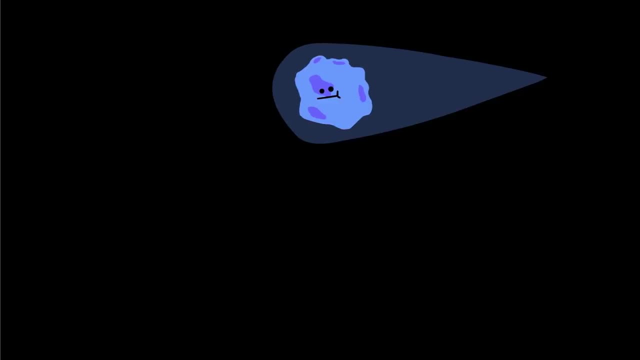 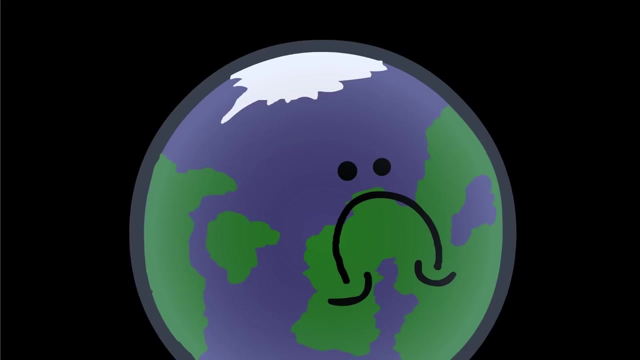 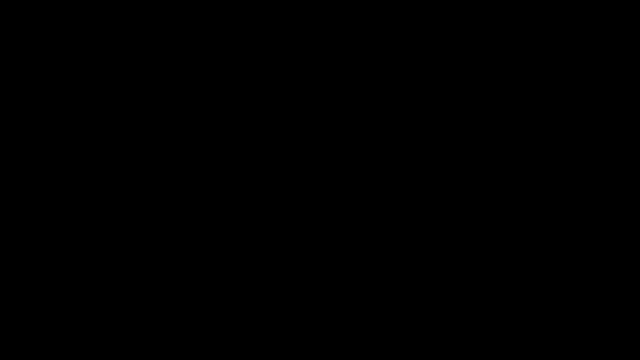 get around Earth. There's space to see. There's planets, comets, asteroids, moons and tons of junk Everywhere- Junk absolutely everywhere to go see and touch and eat. I mean, with all this, who really cares about the Earth? What's an orbit? An orbit is a curved path. 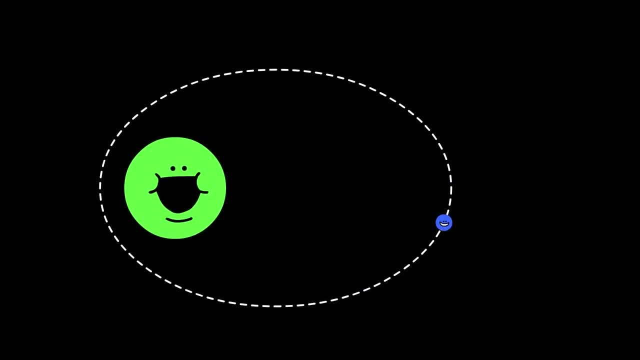 that an object follows around a body, be it a planet, moon or whatever. in space There's lots of different types of orbits. There's low Earth orbits, geostationary orbits, highly elliptical orbits and low Earth orbits. There's also low Earth orbits, geostationary orbits. 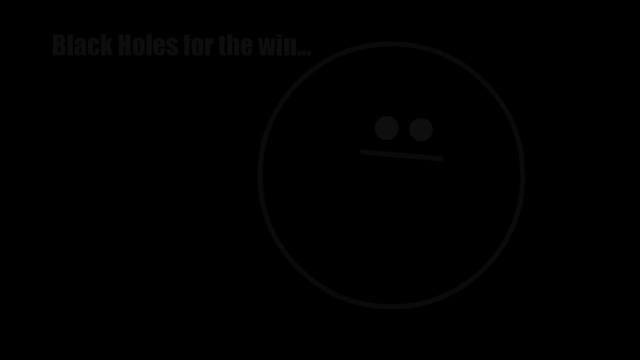 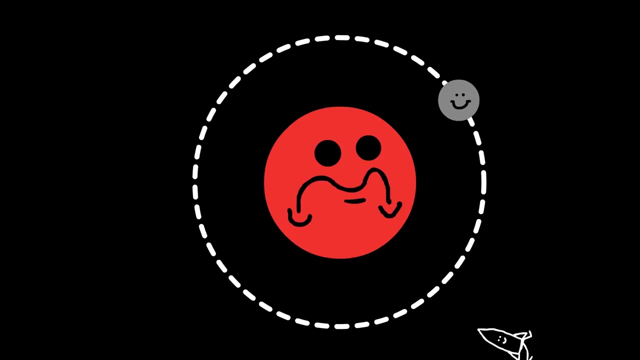 decaying orbits and those freaky-deaky black hole orbits And much more. However, most orbits can be classified as circular, elliptical or parabolic. In a circular orbit, an object orbits a body with a constant altitude and constant velocity. These orbits are really. 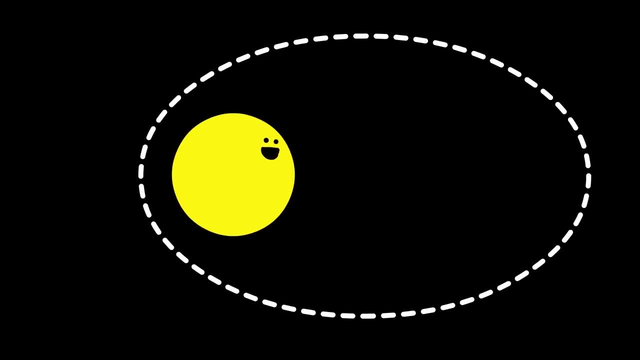 easy to do math with. In an elliptical orbit, an object orbits a body with a changing altitude and velocity on a path in the shape of an oval. An elliptical orbit has an apoapsis and a periapsis. The apoapsis is the furthest point an object is from the Earth and the 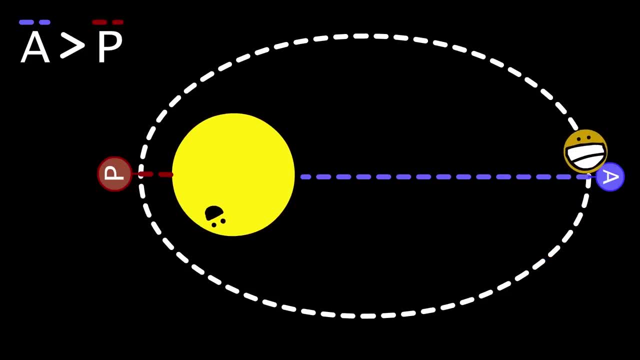 periapsis is the closest point In an orbit. the closer an object is to a body, the faster that object will go relative to the body. So an object moves slowest at apoapsis and fastest at periapsis. The average distance of the periapsis and the apoapsis is called: 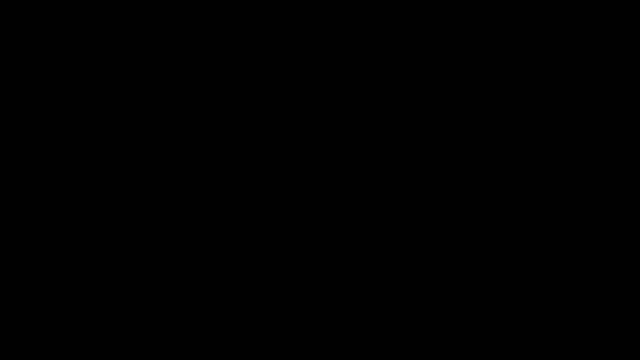 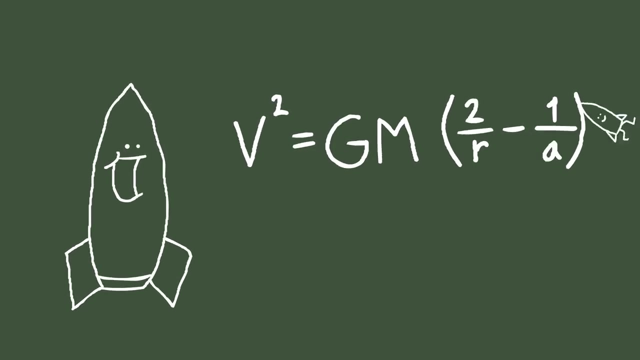 the semi-majoral axis. This value is helpful when doing math. You can find your velocity on any complete orbit with this equation: B is velocity, G is the universal radius and G is velocity. You can find your velocity on any complete orbit with this equation: M is the mass of the body, R is your current altitude and. 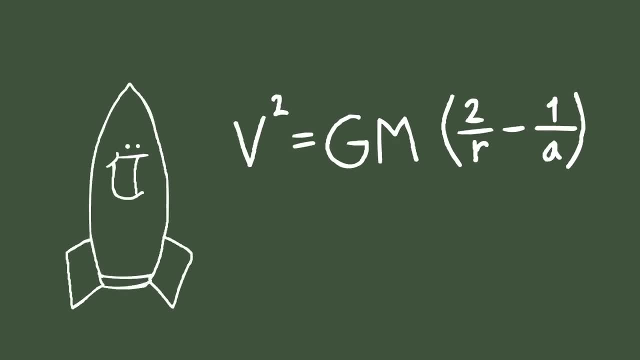 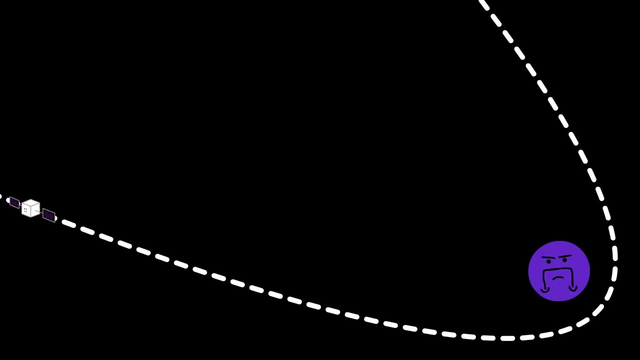 A is the semi-majoral axis, like we saw before. Using this equation and the rocket equation, you can find out what orbits you can achieve with a rocket and how much change in velocity or acceleration is required for each change in your orbit. Lastly, a parabolic orbit is: 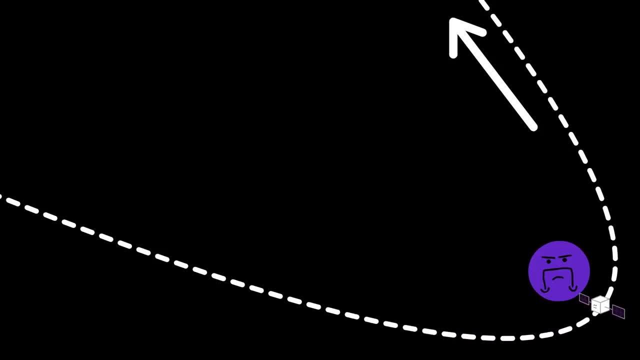 one that an object follows when it is on an escape trajectory from a body. In other words, an object will follow a parabolic orbit if it has enough speed to escape a body's gravitational influence or its gravitational grip. Hyperbolic orbits are a thing too, but they are almost. 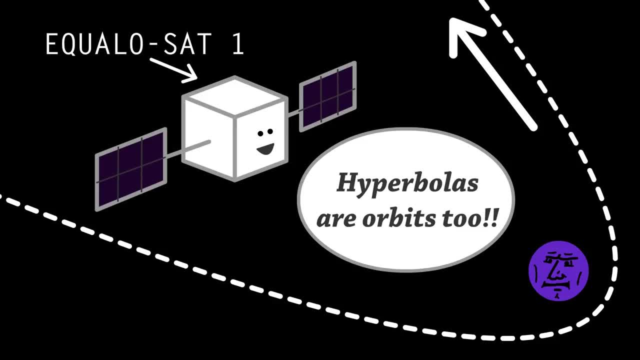 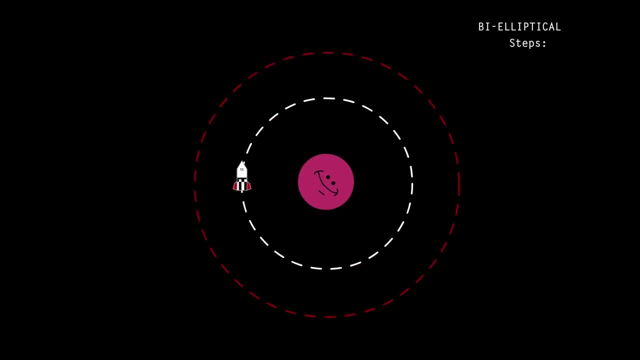 exactly the same as parabolic orbits. Orbits are great and all, but if you wanted to have a different orbit, there are many different ways you can get what you want. First, there is a bi-elliptical transfer orbit. This involves two half-orbits. Basically, you get an extremely 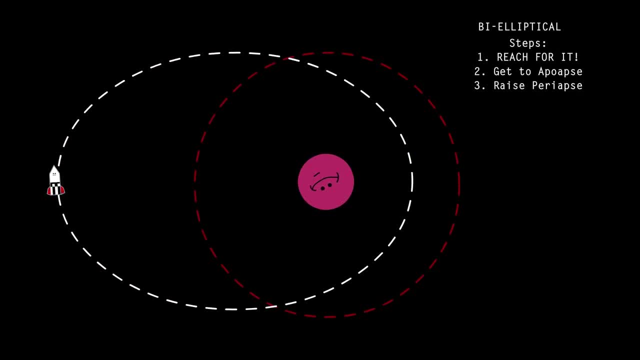 high orbit reach apoaps. change the periapsis of your orbit by accelerating and then correct it when you get to the new periapsis. This maneuver seems a bit ridiculous, but it can be extremely efficient And, believe it or not, sometimes it is even more efficient to. 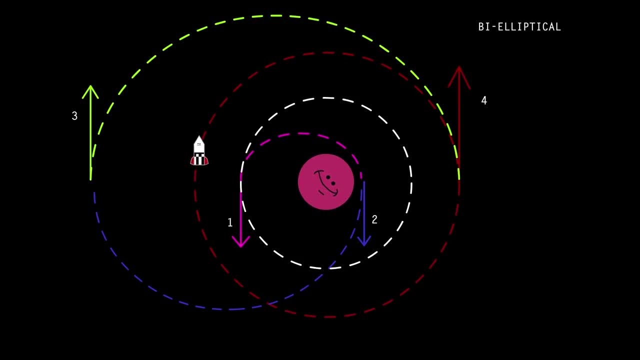 slow down a rocket and achieve a new apoapsis from an even lower periapsis. Second, there is a Hohmann transfer orbit. This is much more direct. First you accelerate and change your apoapsis. then you accelerate again at the new apoapsis, giving you a new 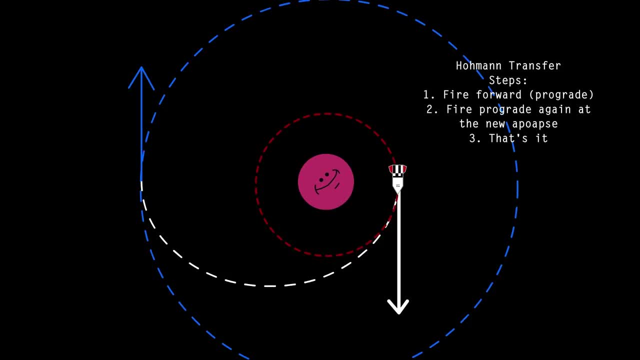 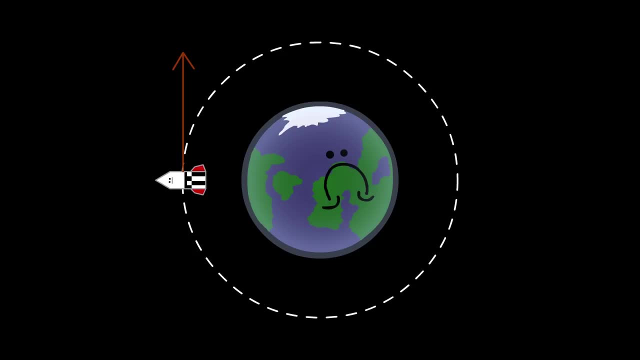 circular orbit. That's about it. Almost all transfer orbits are done this way or with gravitational assists. You can't effectively change an orbit by firing away from a body. This will change your radial That thing. It's not effective or efficient, so don't. 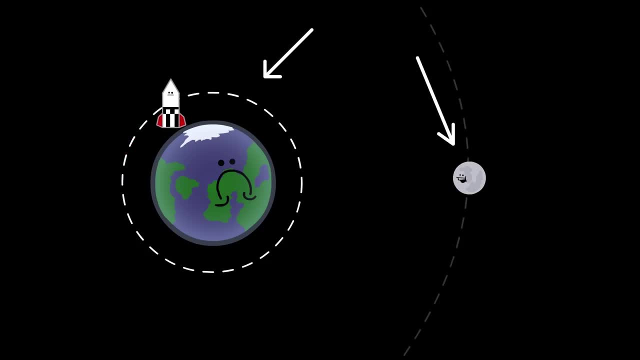 do it. Let's apply this: Here's the earth and here's the moon. Right now, we're orbiting the earth and we need to get to the moon. How are we going to get to it? Simple, In a straight line. Wait a second. that's not a path to the moon, that's a colli- oh, oh. 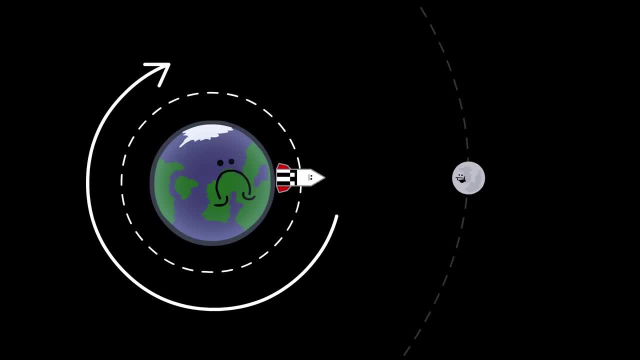 All right, let's try that again and think in motion. Right now we're removing the planet like this and we need to get to that. What direction should we move and when? to get to that? You might think it's best to shoot for the moon when you're the closest. 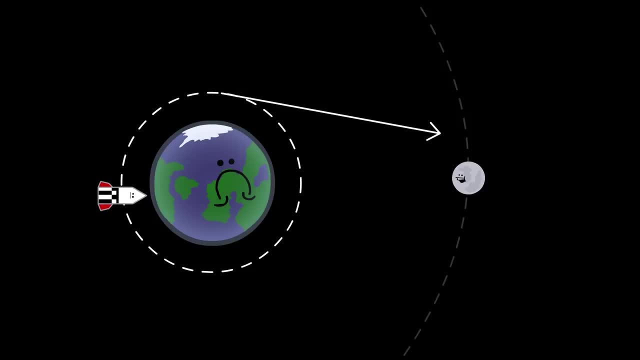 but that's not the case. It's way more complicated. If we fire our engines here enough, we will eventually make it to the moon, but the speed we'd have to be running at would send us sailing past the moon. If we fire our engines here, we can get to the moon much easier, and 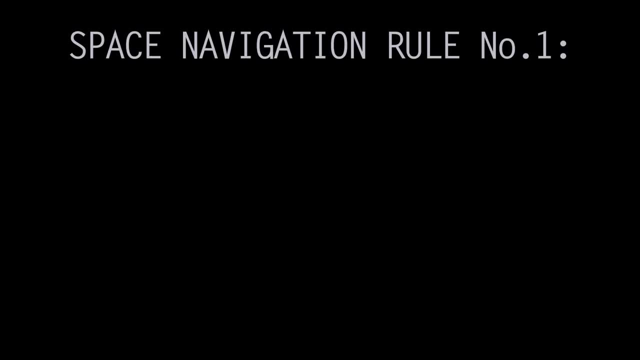 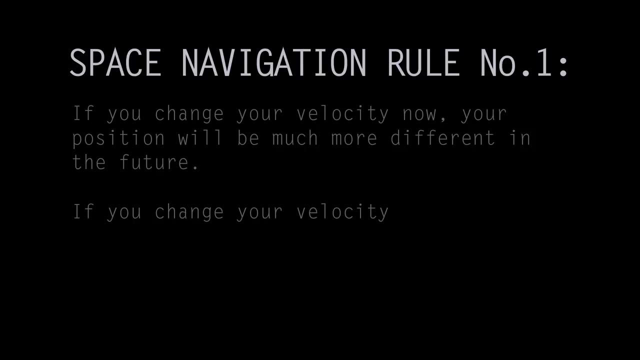 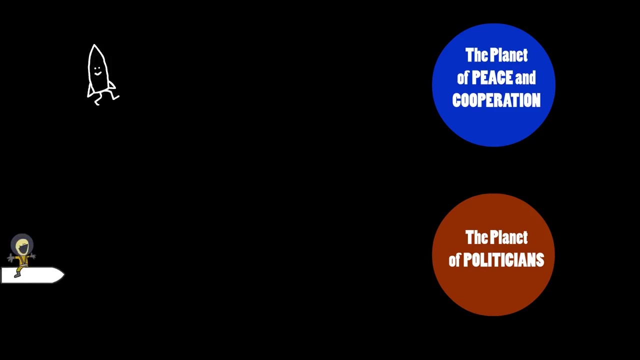 with much less fuel. Space navigation rule number one: If you change your velocity now, your position will be much more different in the future. If you change your velocity later, your position will not be as different. That's a life lesson and a physics fundamental. If you need to change direction to get to something in space. you can change direction with much less fuel, the further you are from that object. If you need to get to Mars and are here going this way, you can burn for ten seconds now, go right for it, or burn a hundred days later for well over ten seconds. 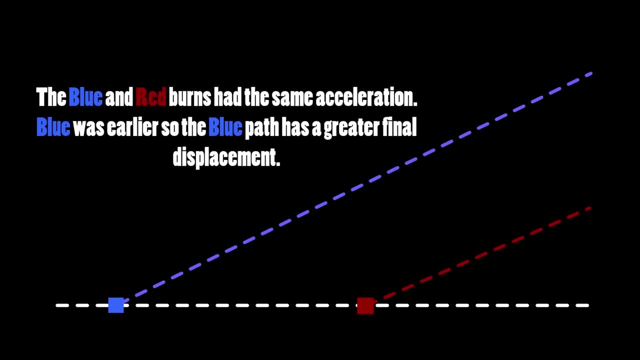 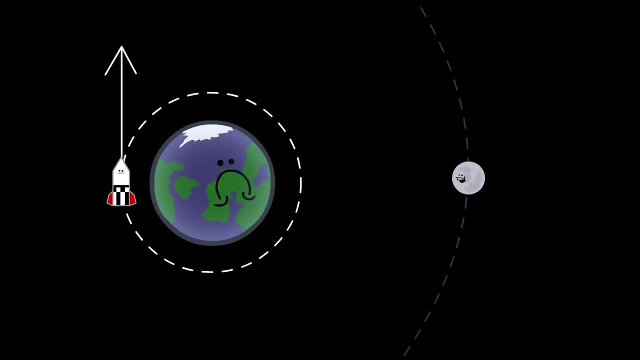 But you can still never get to Mars. This works on linear paths, so it has to work on curved paths. So with this logic, if we burn here, we can get to the moon with the least amount of fuel. Awesome, We can finally do it. 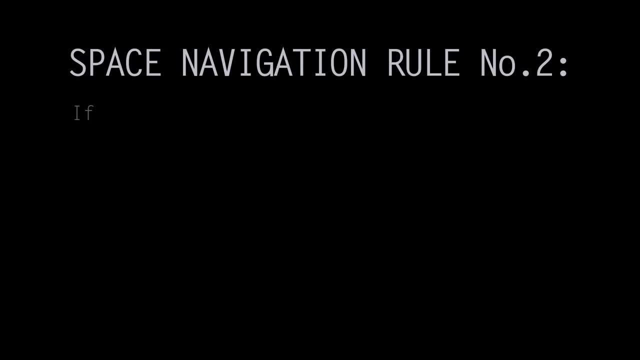 Yu- WHAT Space navigation, rule number 2.. If you're going to go to space, know where you're going. If you know where you're going, know where that place will be when you get there. If not, you're either going to die or find something that will shock the world to its 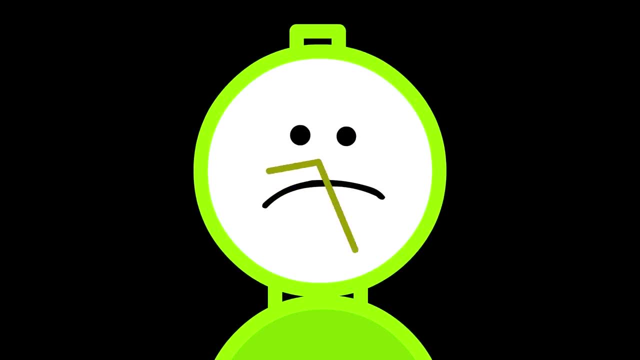 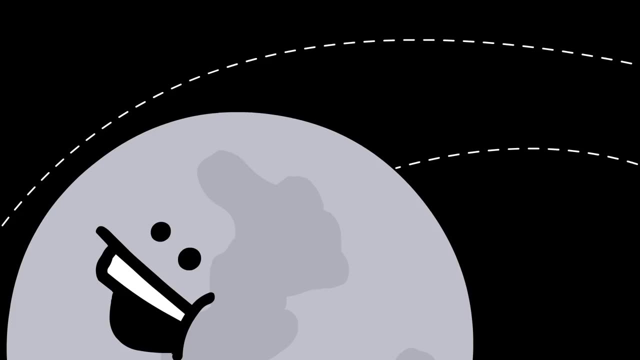 core, If you were alive, to tell the world about this. Keep in mind that you don't need perfect timing to get to the moon in one shot. There are many other ways you can approach it. Also, don't forget, if you set up an orbit to get to the moon, make sure that when you 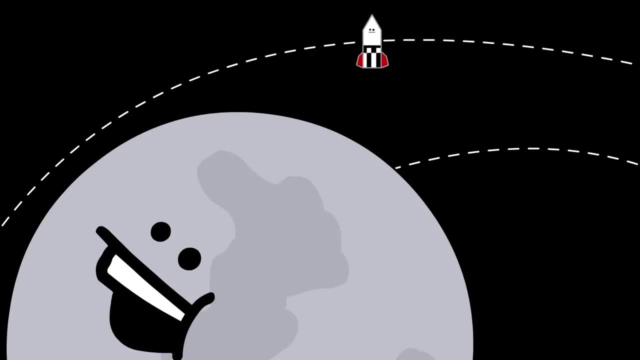 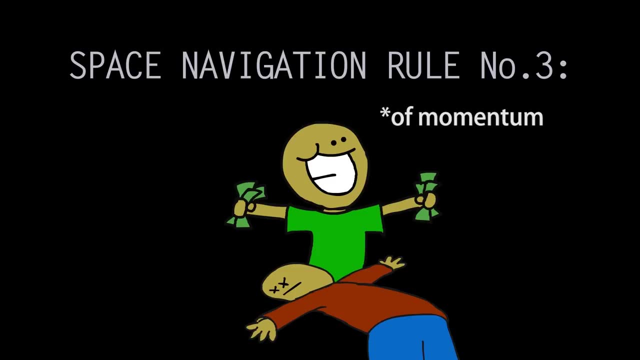 end up orbiting the moon. it's at a safe altitude and velocity. Aim to orbit the moon, not to make a crater Space Navigation. Rule Number 3. Loot Bodies. That's right. you can literally steal momentum from other bodies in space. 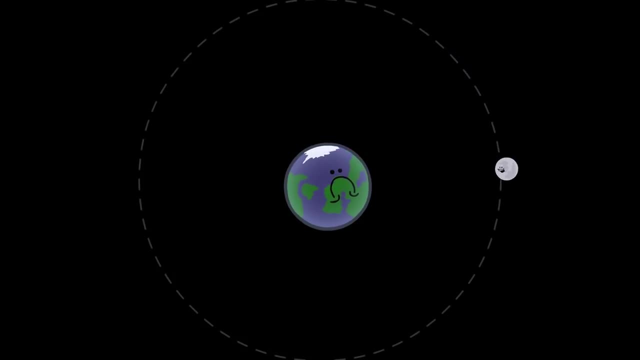 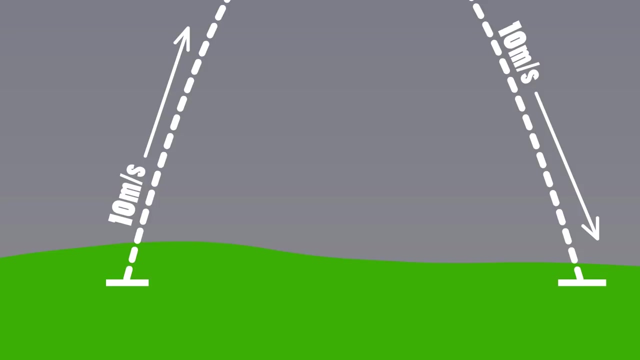 Because of the moon. it's orbiting Earth which we are going to leave. How can the moon help us? Let's start with a simple idea: behind gravity, What goes up must come down. If something goes up at a certain speed, it will come back down at that exact speed at. 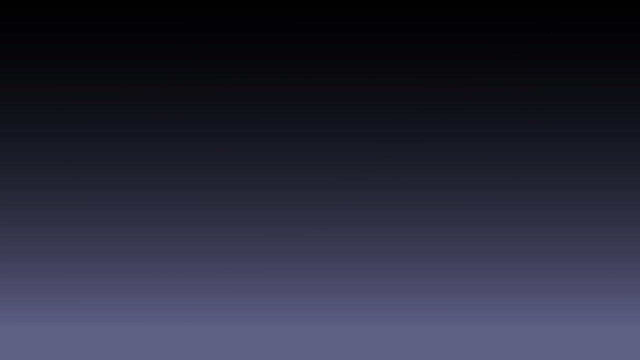 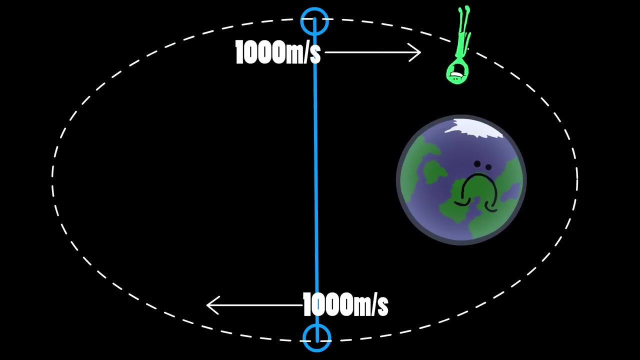 the initial launch altitude. This is the same for orbits. If an object is moving a thousand meters per second on one side of the Earth, it will be traveling a thousand meters per second when it reaches that same altitude on the other side. So let's say we have Stan the Satellite orbiting the Earth with an orbit slower than the moon's. If the moon passes Stan close enough to the moon, it will be able to fly to the moon. If the moon passes Stan close enough to the moon, it will be able to fly to the moon. If the moon passes Stan close enough to the moon, it will be able to fly to the moon. 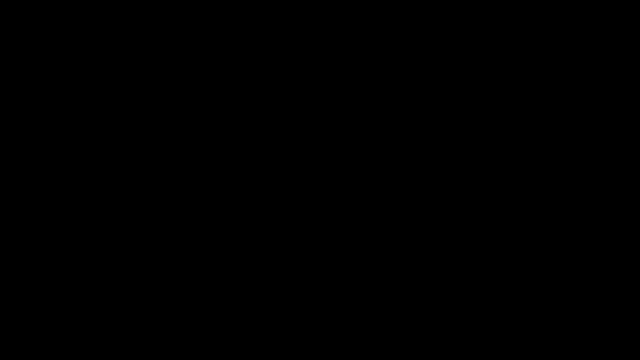 If the moon passes Stan close enough to the moon, it will slingshot Stan around itself and forward, giving Stan a much faster velocity than before. Since the moon was moving faster than Stan, Stan fell towards the moon, then around it and finally away from it.